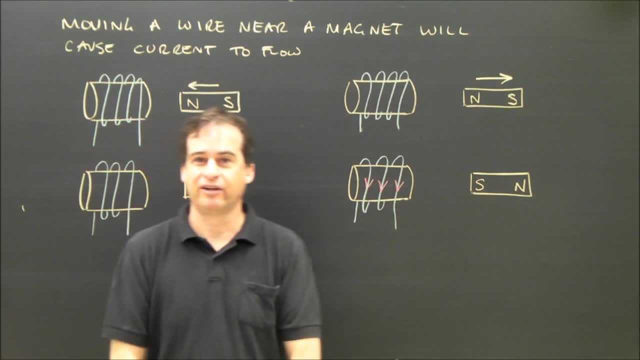 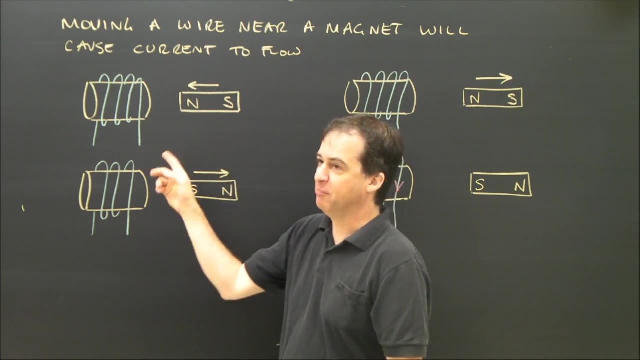 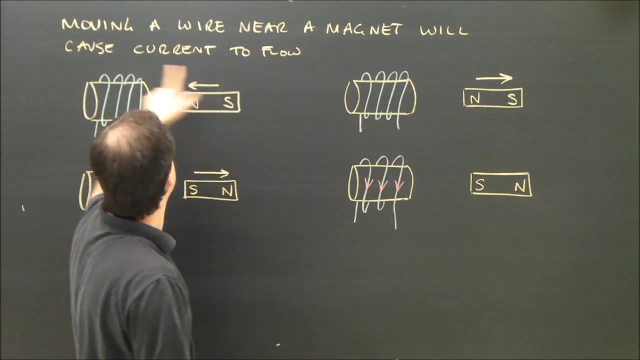 Okay, what we're going to look at is how we generate electricity. Okay, so what we want to do- this is called Lenz's Law- is figure out when a magnet is moving near a coil, which way will electricity flow? First thing you've got to remember is: moving a wire near a magnet will cause the current to flow, or moving the magnet near the wire. Either way, if the two are moving near each other, you're going to get electricity to flow. The question is: which way is electricity flowing? And, as I said before, as I said before, if you're going to get electricity to flow, you're going to get electricity to flow. So, if you're going to get electricity to flow, you're going to get electricity to flow. So, if you're going to get electricity to flow, 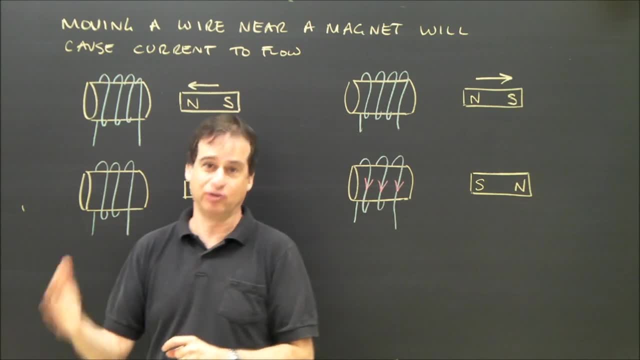 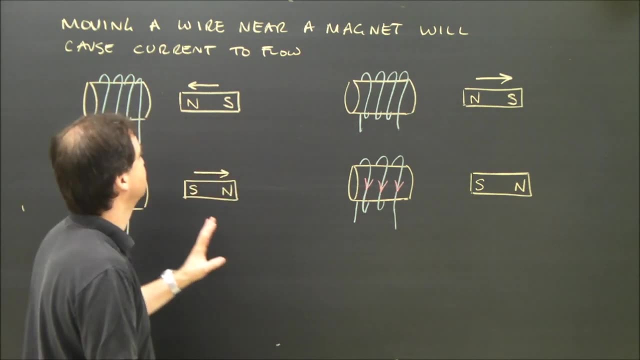 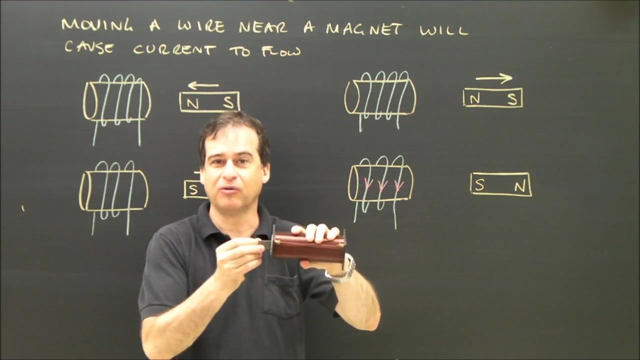 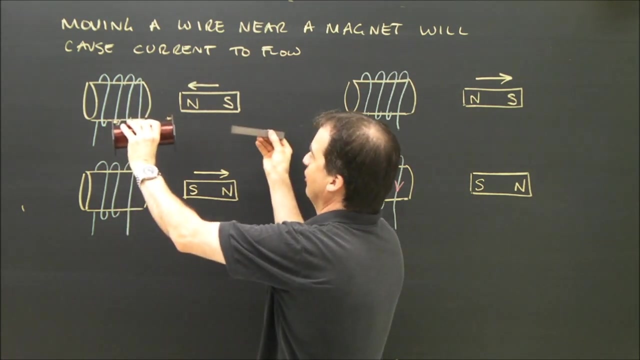 the other videos. if you're told to use the right hand rule, use the right hand rule. you'll get the appropriate answer for the right hand rule. If you're supposed to use the left hand rule, use the left hand rule, you'll get the appropriate answer. So let's take a look at this. I've got a magnet moving near a coil. When electricity, when a magnet is moving near a coil, in or out of a coil, it will cause electricity to flow in that coil And we want to know which direction it's flowing. So I've got a coil here, I've got a magnet and the north is going into the coil And I'm not going to get into a big 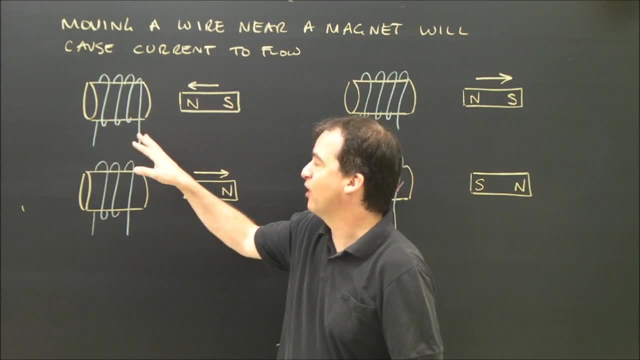 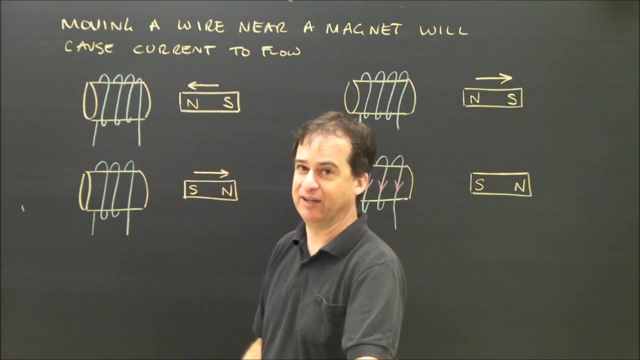 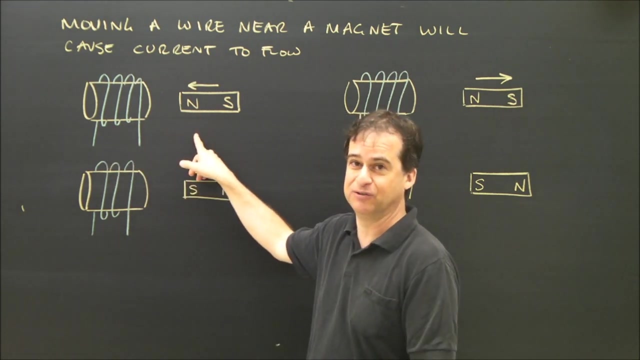 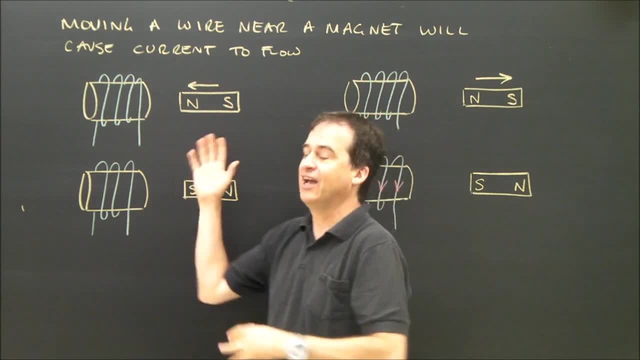 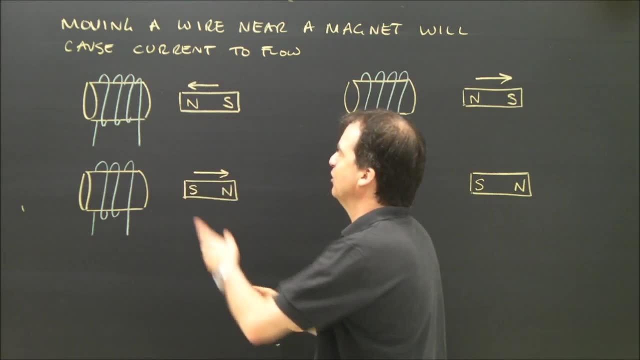 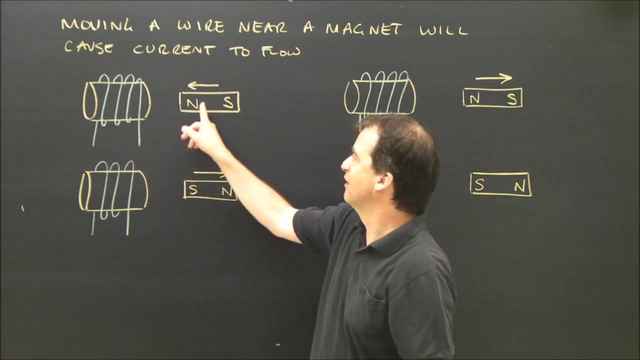 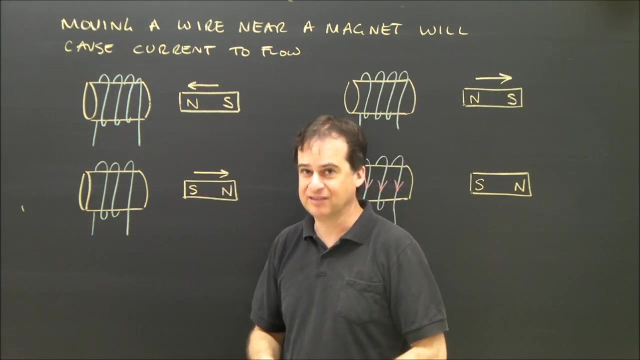 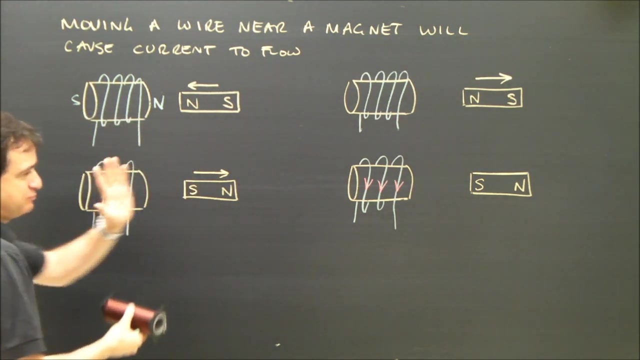 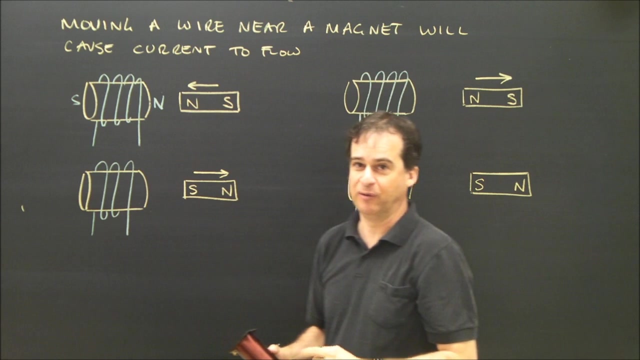 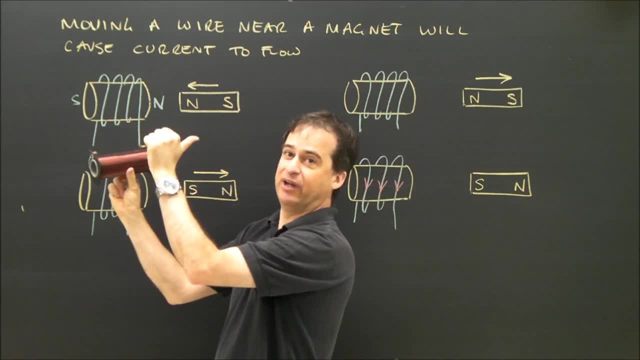 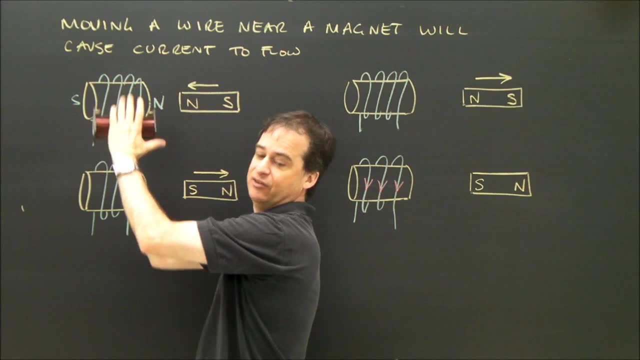 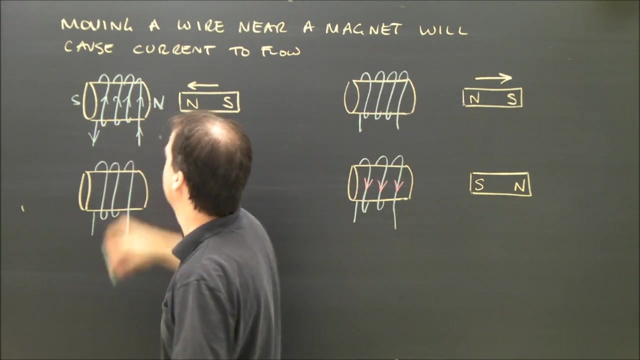 in such a way that my thumb points to the right and my fingers point in the direction of electricity flow. I put my thumb like that. the electricity is flowing up on the top of this coil if I use the left hand rule. So it's going this way: Up here and down there. 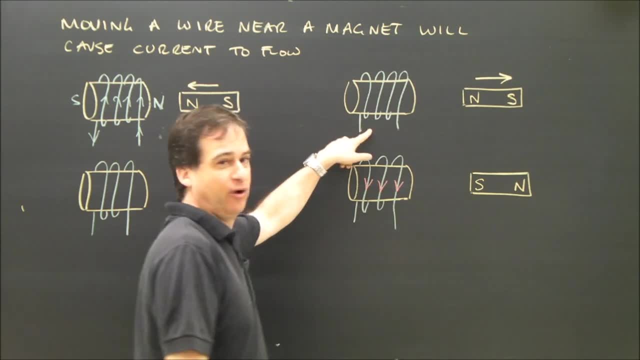 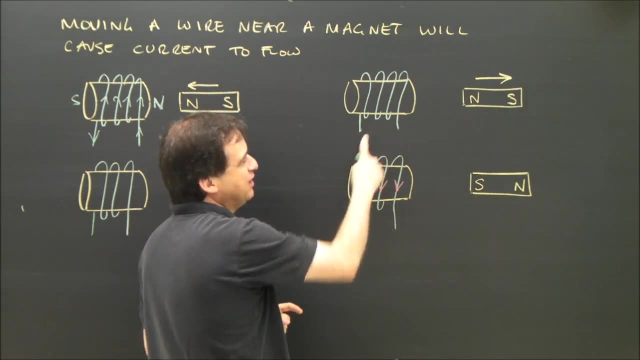 Let's try another one. Here's another coil. I'm taking my magnet and this time I'm pulling the magnet out. How can I make that difficult? Electricity is going to flow in here in order to make the poles of this. make this difficult. 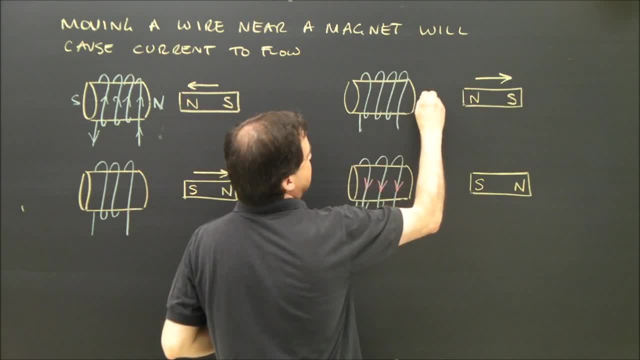 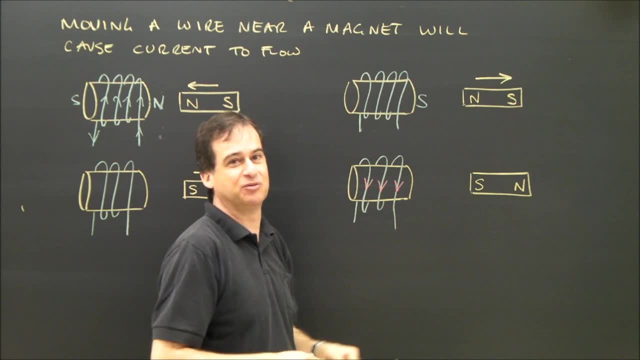 Well, if I'm pulling the north out, if this is south, then that south is trying to pull the magnet back in And I'm pulling the magnet out. It's making it difficult. That's the way the rule works. So this is south, this is north. I treat it like an electromagnet. 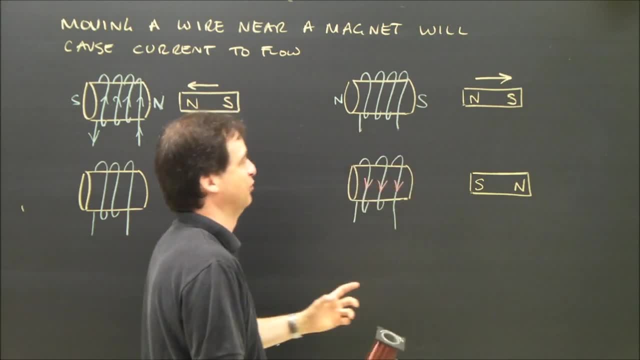 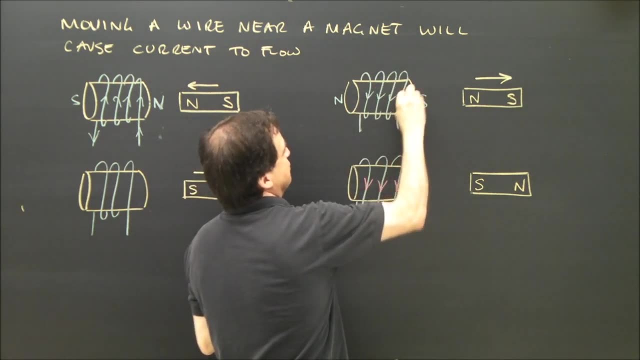 If this is north and this is south in a coil, which way is electricity flowing? So I'm using the left hand rule. Put my thumb this way, grab it. My thumb goes this way. My fingers are down in the front, So they must be. the electricity must be flowing that way. 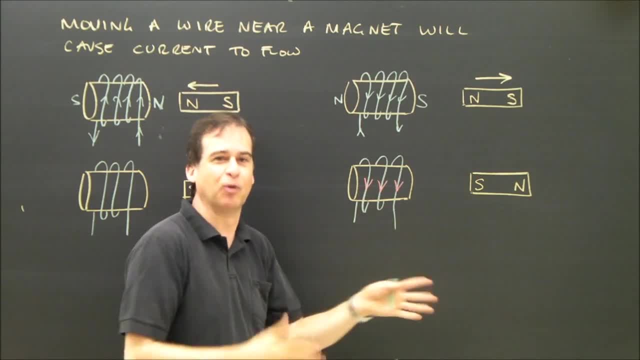 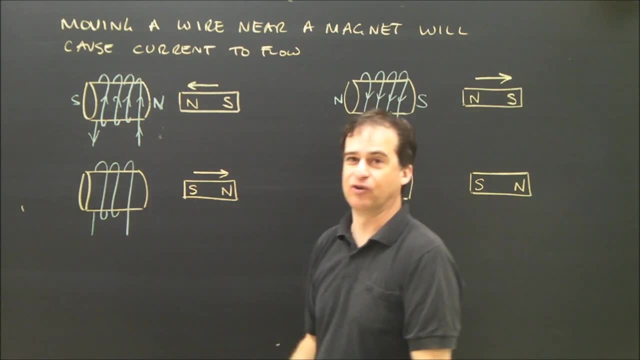 If I'm using the right hand rule, I get a different answer, but it's appropriate for the book I'm using. Okay, Let's look at a third one. This is a south being pulled out of a coil. If a south is being pulled out, I need to make this a north. 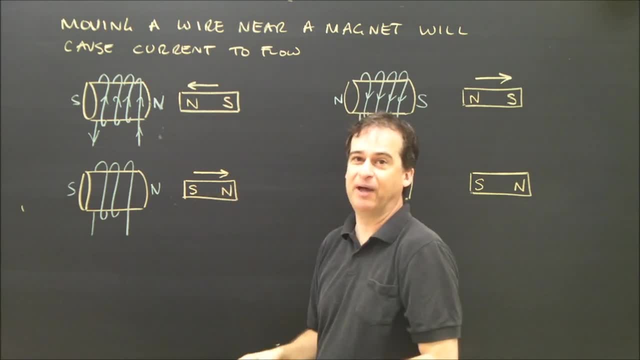 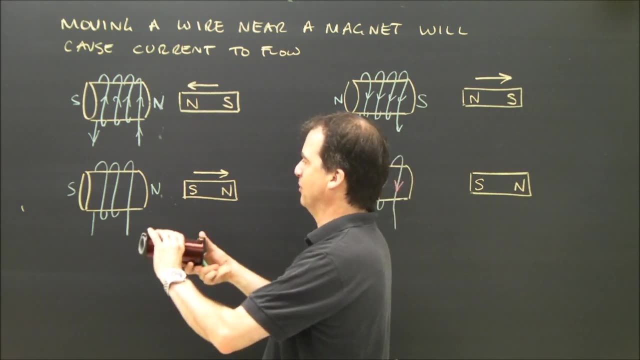 The reason is this north is trying to pull this south back in and I'm trying to pull the south out. That's making it difficult. So this is a north and this is a south. I got my coil. My thumb's got to point to the right. 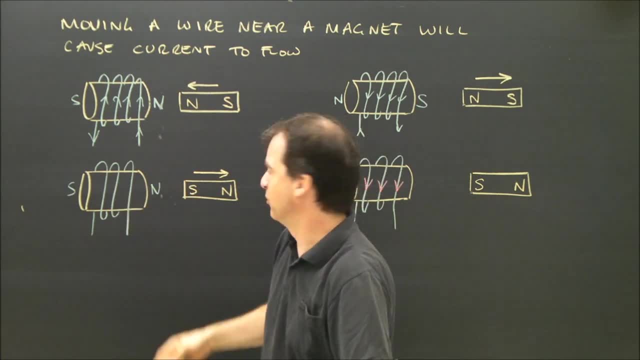 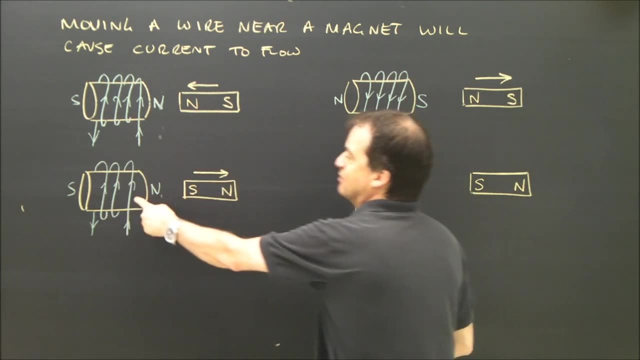 My fingers, therefore, are going up. Since my fingers are going up, the current flow is that way. So when I do this, this is the way the current's going to flow. Let's look at this one here. I know the direction the current is flowing. 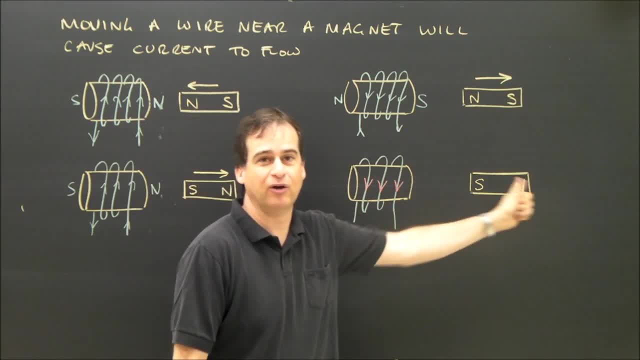 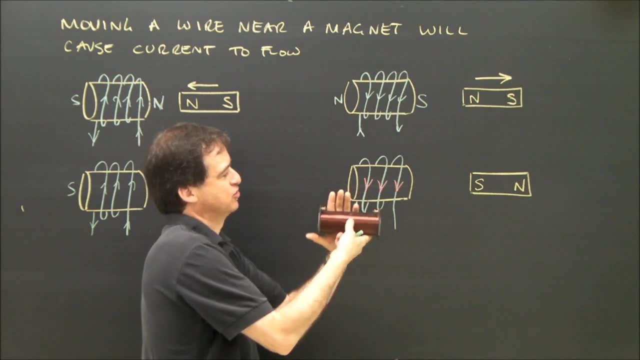 I got my magnet and I want to know: is the magnet being pulled out or pushed in? So I go here. I know the direction of the current. My fingers go down on front. My thumb is therefore to the left. So this must be a north and this is a south. 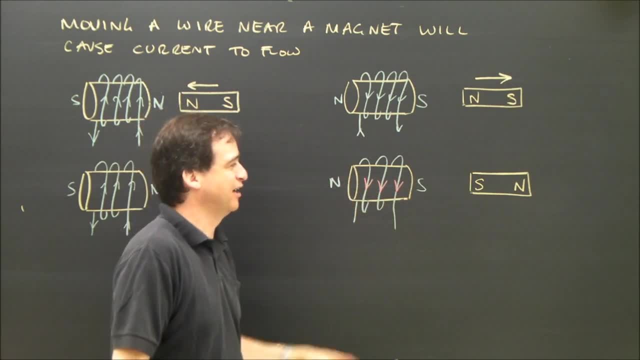 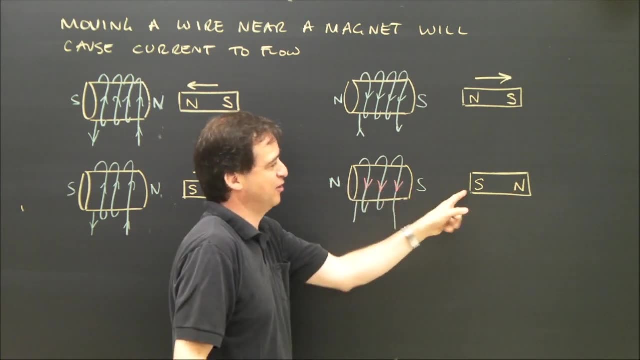 This electromagnet. this is north, this is south. I'm generating that curve by moving this magnet. Which way am I moving it? If this is a south and this is a south, they're repelling This south, is trying to push the magnet out. 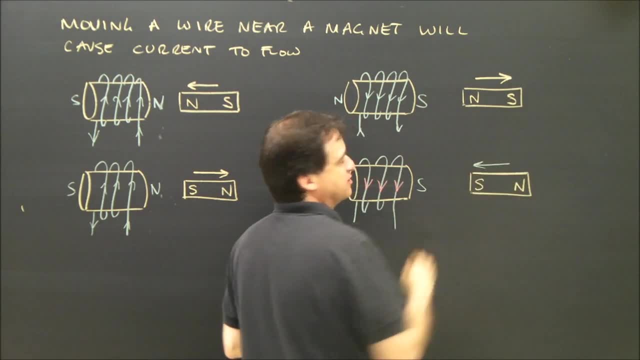 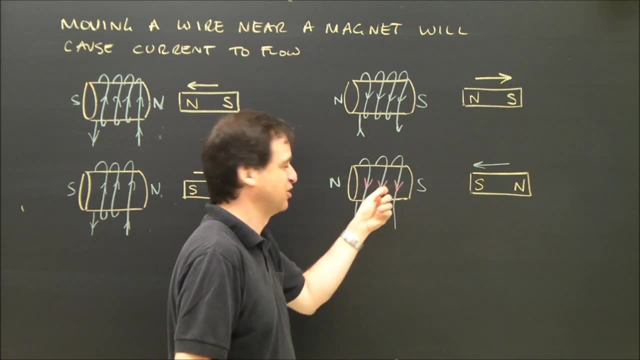 I've got to do the opposite. That's making it difficult. If this south is going in, This south is going in and this is south. That's making it difficult for me to push this in, because it's repelling And, as a result, electricity will flow that way. 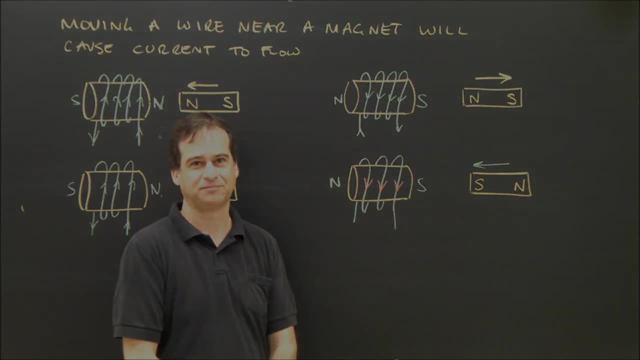 So you can do it either way. I hope that helps. 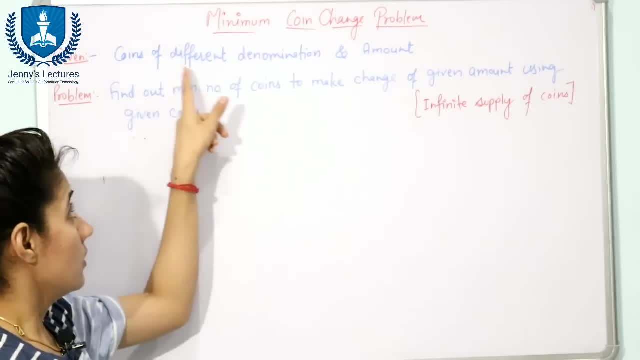 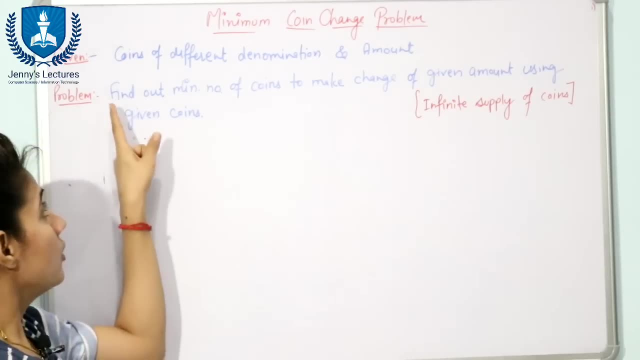 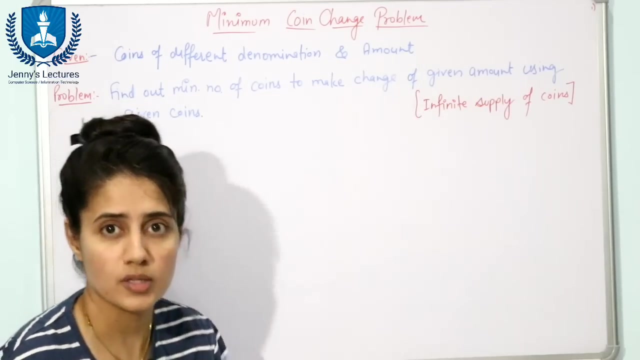 We will discuss what We are given, what Coins of different denominations and certain amount would be given. And now what you have to find out. The problem is what You have to find out: minimum number of coins to make the change of given amount using the given coins. Okay, How this problem is.